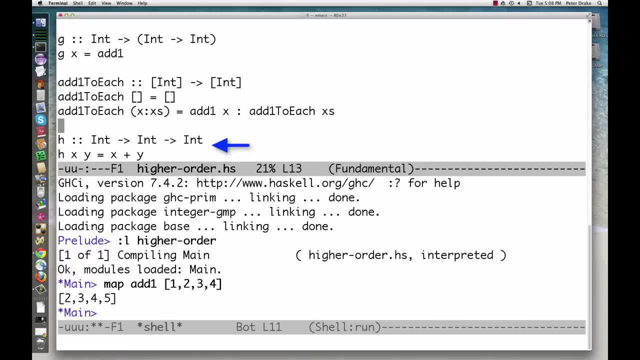 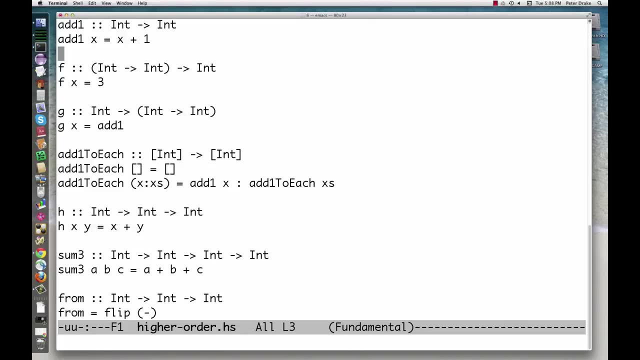 Now consider this function. So far, we have imagined that this function takes 2 ints and returns a third one, but that's not really what's going on. Take a look at the type signature. If the arrow associates from left to right, then h has the same type as f. If the arrow 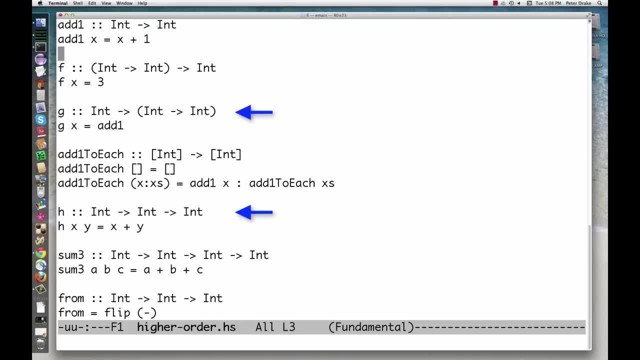 associates from right to left. then h has the same type as g. It must be one of the two. It turns out that it's the second one. h takes an int and returns a function that in turn takes an int. It returns the function. 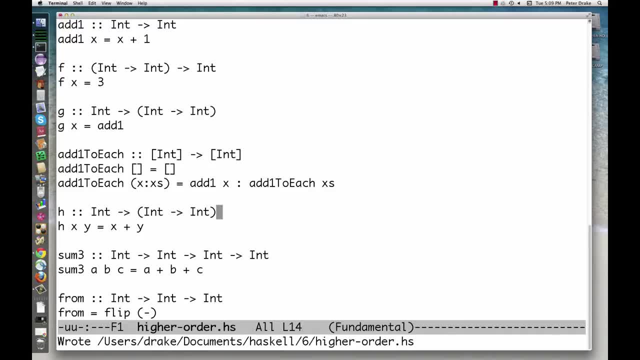 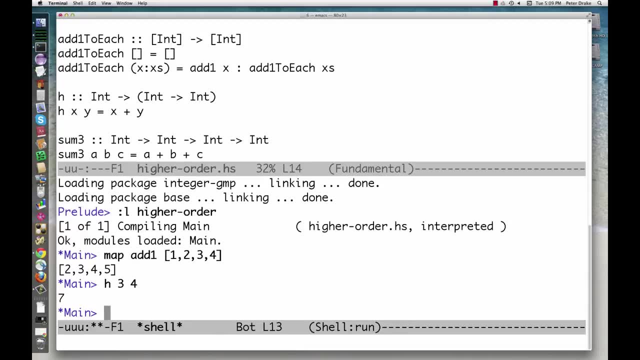 an int and returns an int. Now, wait a minute. We know that this function is perfectly happy to take two ints. What's going on Again? think about associativity. This is the same as either h of three of four or h of three of four, Asking for three of four in the second. 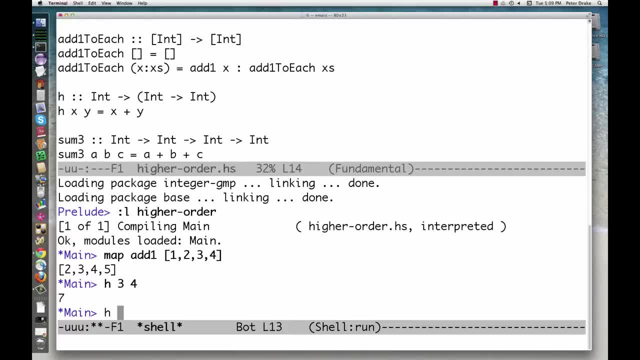 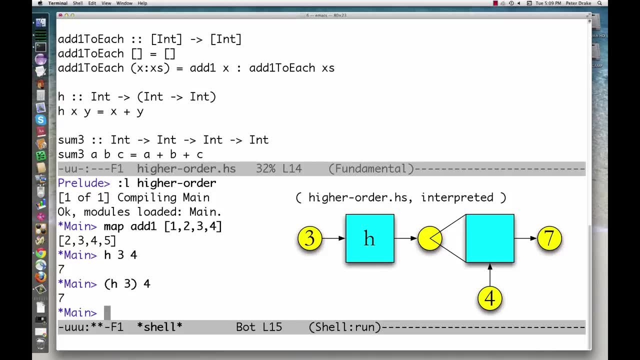 case doesn't make any sense, so it must be the first one. We take h of three, which returns a function, and apply it to four. So what function is returned? when we ask for h of three, We get an error message. but Haskell is not telling us that taking h of three is. 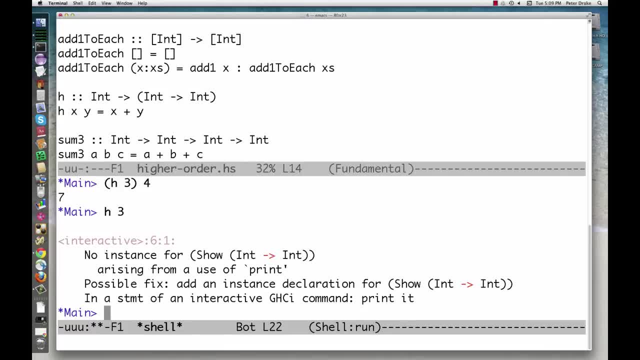 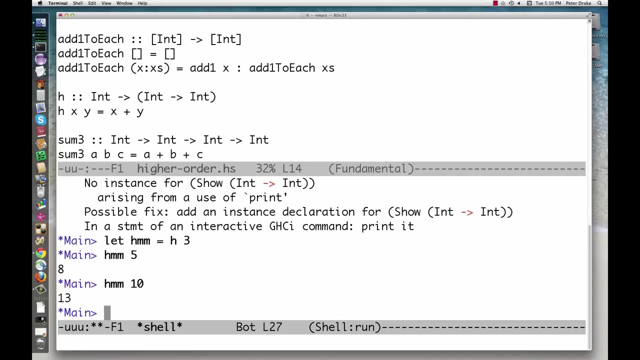 illegal. Haskell is just saying that it doesn't know how to print the resulting value, which is a function of type three. We can store this value in a variable. Now we have a function that we can apply to a number. The function hmm then adds three to its argument. It is the result of partially 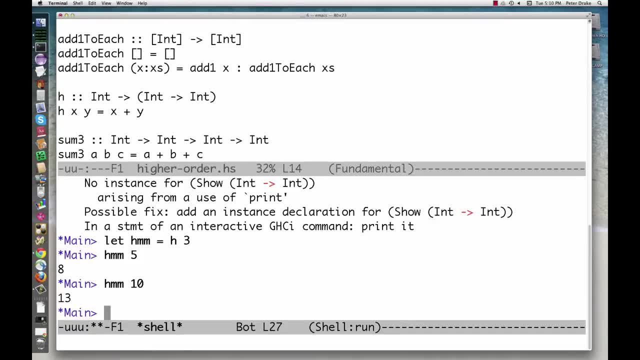 applying the function h. Any Haskell function that appears to take multiple arguments can be partially applied this way. Here we partially applied max to get a function that returns the max of three and its argument. We then mapped that function, which has no name, over a list. In fact, every Haskell function takes one argument and returns one. 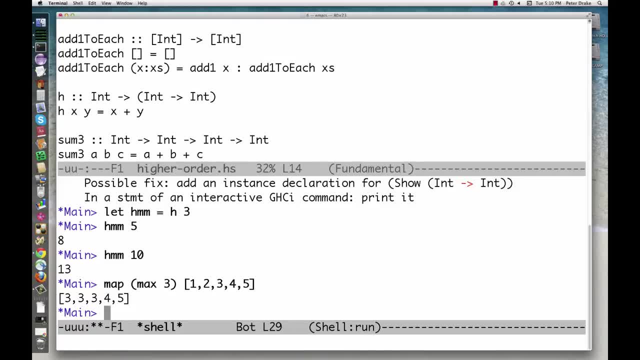 value. If it appears otherwise, it's because applying the function really involves creating a series of functions and applying each one to the next value. The type here could be written as: SUM3 takes an int and returns a function. That function takes an int and returns another function. 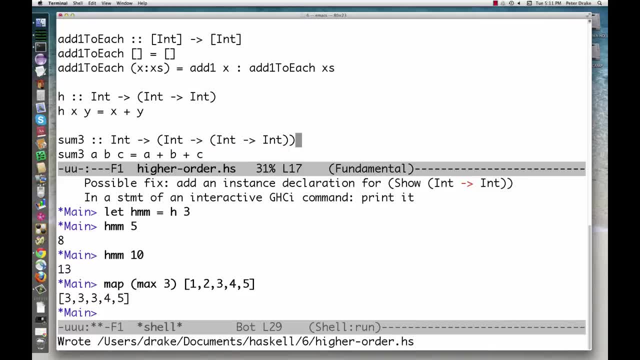 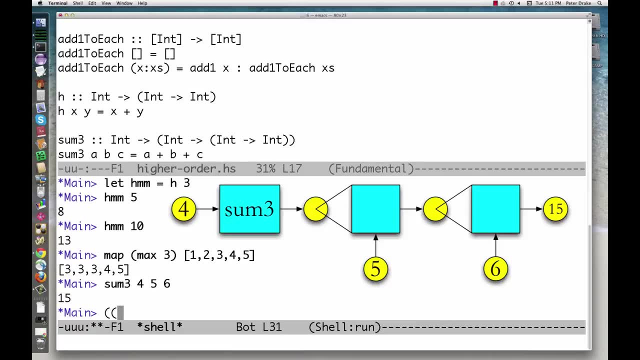 That function takes an int and returns an int. When we ask for, we are really asking for. Haskell allows us to leave out the implied parentheses in both the type signature and the function application. Functions that are broken down like this are said to be curried after Haskell curry. 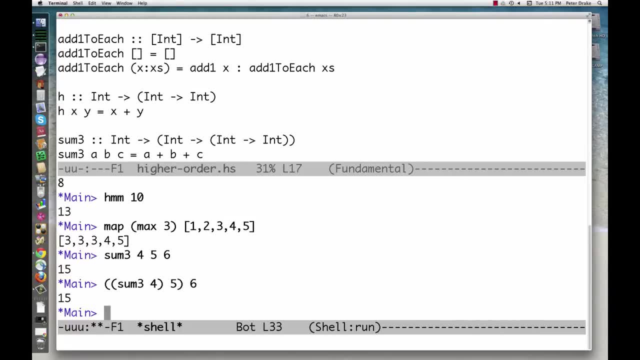 Currying is possible in all functional languages. In Haskell all functions are automatically curried. InFix operators are also curried. Conveniently, we can supply either of the two arguments. MAP is built in, but it could be defined like this: 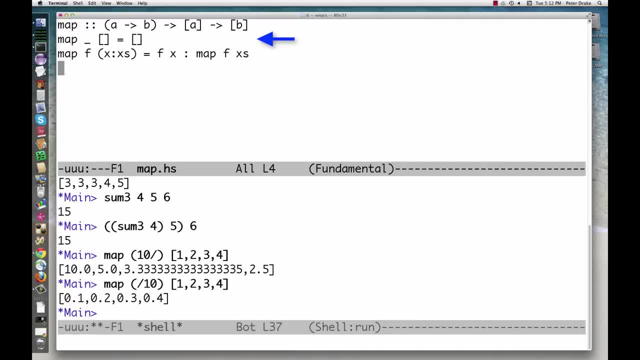 Strictly speaking, because it is curried, MAP takes a function from A to B and returns a function from a list of A's to a list of B's. Most of the time, it's easier to imagine that it takes two arguments: a function and a list. 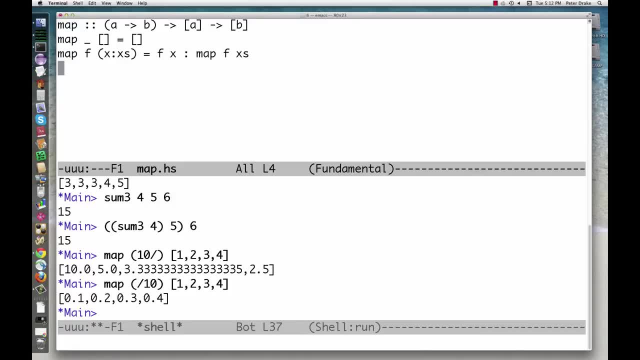 and returns a list. We'll often talk about functions as if they take multiple arguments. Just remember that we could partially apply them if we really wanted to. Now suppose we have two lists that we want to combine with some function. The higher order function, ZIPWIDTH, makes this a snap. 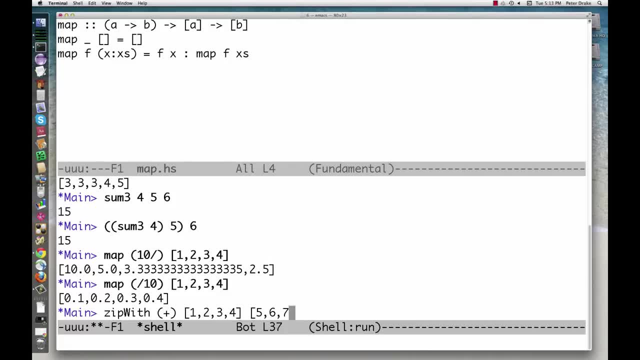 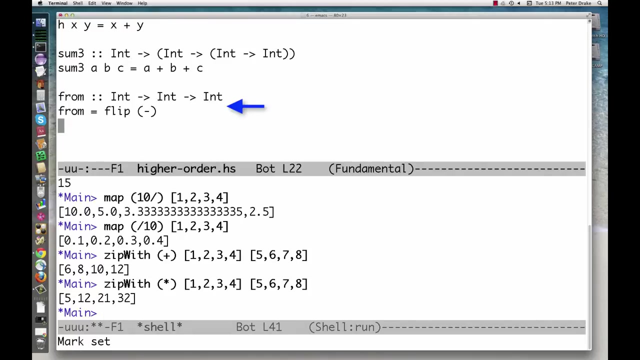 To get a function that's just like an existing one, but with the arguments in the opposite order, use FLIP. This says that FROM is the result of flipping the subtraction operator. FILTER takes a function and a list and gives us a list of those elements for which the